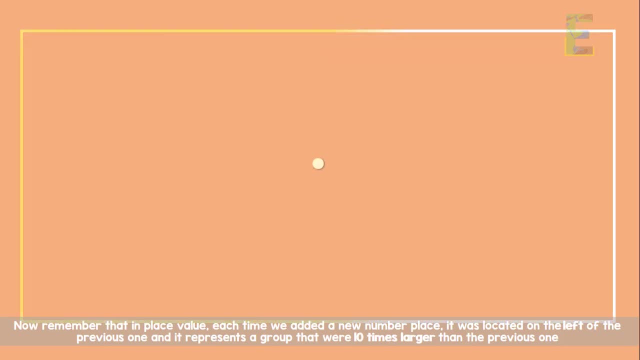 Now remember that in place value, each time we added a new number place, it was located on the left of the previous one and it represents a group that were 10 times larger than the previous one. So since the amount gets bigger and bigger as we go to the left, then we can also say: 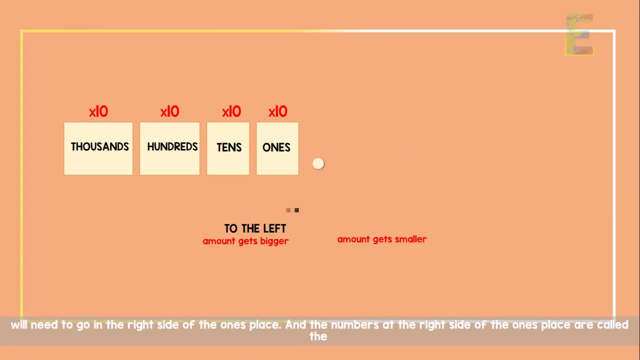 that the number place for counting smaller amount will need to go in the right side of the ones place. Okay, And the numbers at the right side of the ones place are called the decimal numbers. Decimal numbers and whole numbers are separated by a reference point called decimal point. 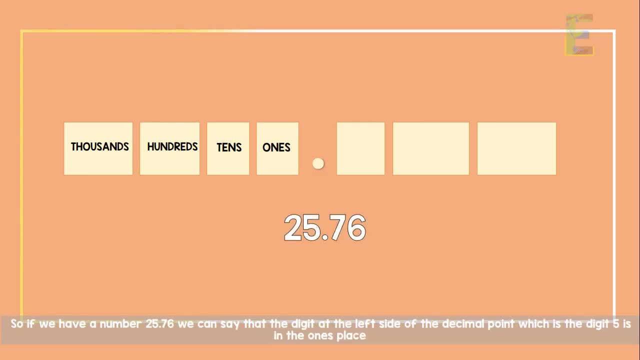 So if we have a number 25.76, we can say that the digit at the left side of the decimal point, which is the digit 5, is in the ones place. Now, how about the number at the right side of the decimal point? 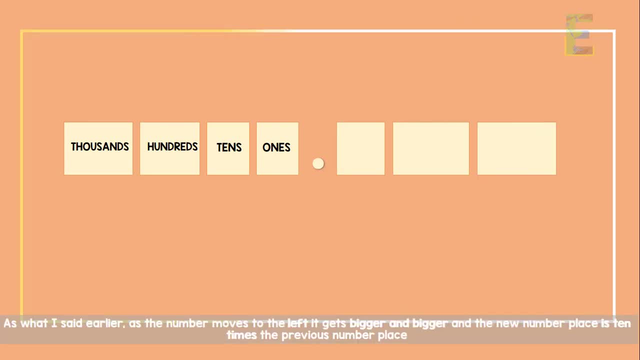 What are the names of those digits? As what I said earlier, the digit 5 is in the ones place. As the number moves to the left, it gets bigger and bigger and the new number place is 10 times the previous number place. So each time we move to the right the number place are 10 times smaller than the previous place. So the digit at the right of the decimal point is called the tenths place, meaning it is the one tenth place. The decimal numbers keep going to the right and each time new number place is added to. 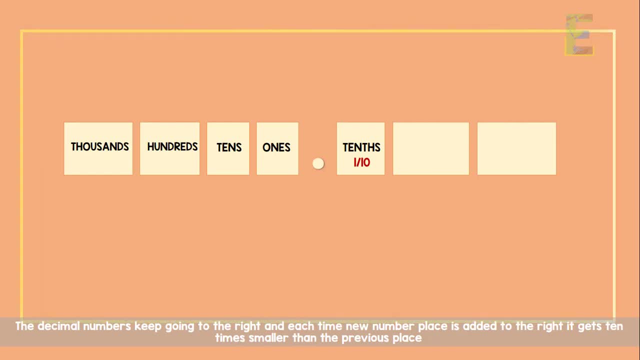 the right, It gets ten times smaller than previous 123.. Therefore the next number is called the hundredths place, which means one over 100, and next number will represent the one tenths of 100, which is the one thousandths, and so on. 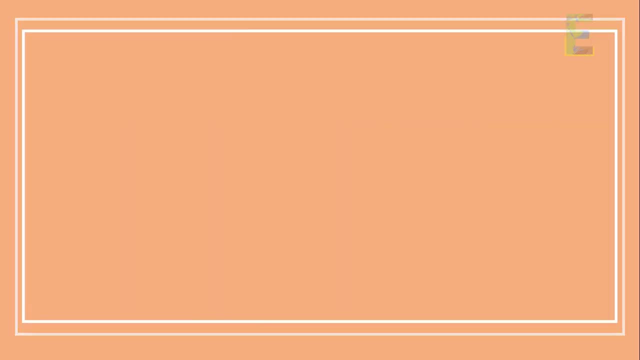 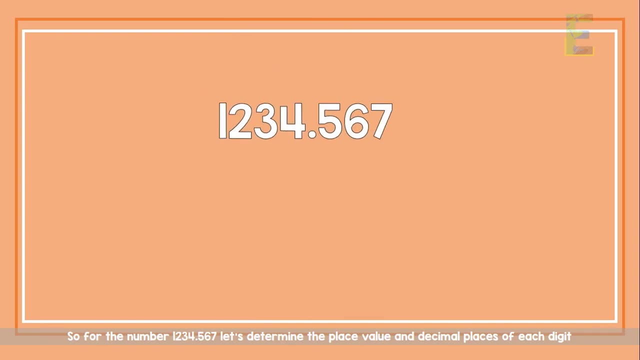 An example of a decimal number: 1.234.567.. Let Display, Let's see it- 1.2234.567.. determine the place value and decimal places of each digit. The numbers on the left side of the decimal point are the whole number and the numbers at the right side of the decimal 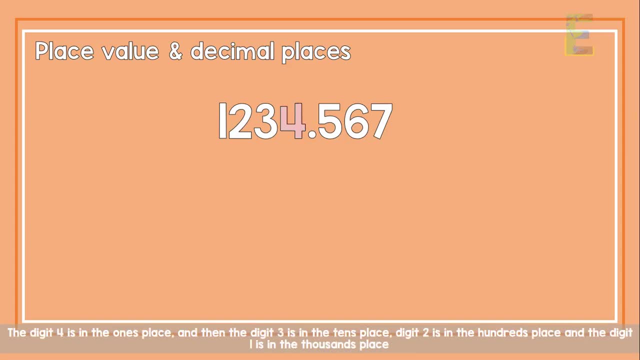 point are the decimal numbers. The digit 4 is in the ones place and then the digit 3 is in the tens place, Digit 2 is in the hundreds place and the digit 1 is in the thousands place. Now for the decimal numbers. digit 5 is in the tens place, then digit 6 is in. 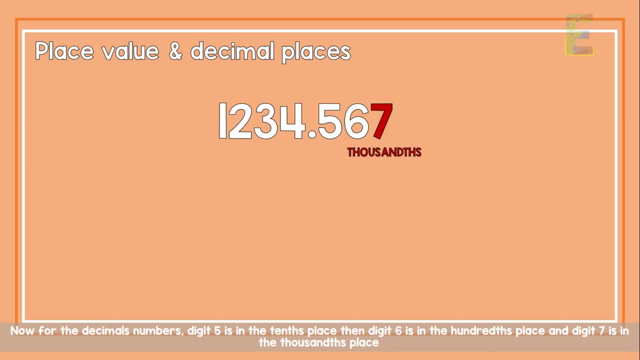 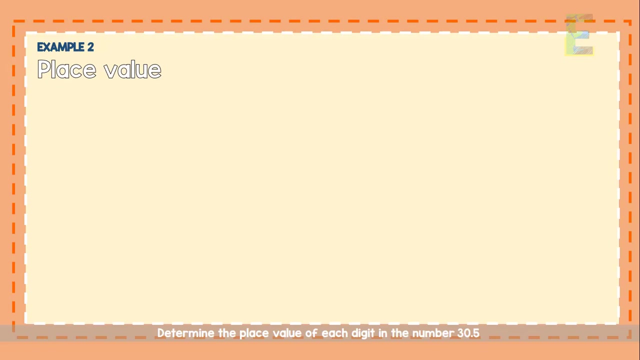 the hundreds place and digit 7 is in the thousands place. So if we expand this number, it will look like this, And if we add these 7 values, we will get 1234.567.. Now let's have another example: Determine the place value of each digit in the number 30.5.. As 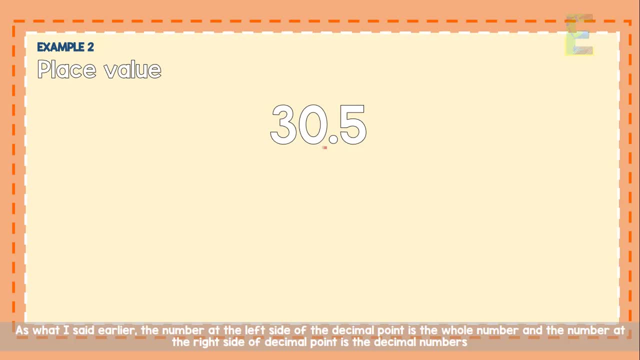 what I said earlier. the number at the left side of the decimal point is the whole number, and the numbers at the right side of the decimal point are the decimal numbers. The digit at the left side of the decimal point is in ones place, which, in this problem, is the digit 0 and next. 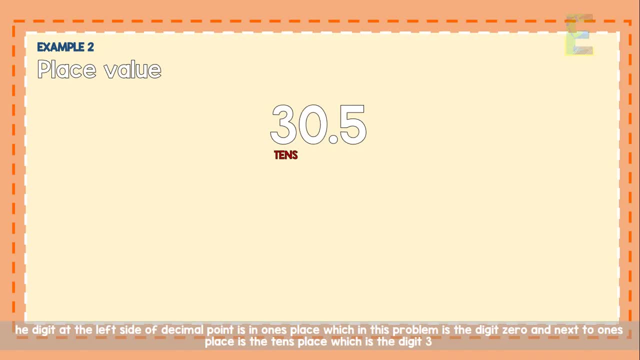 to ones place is the tens place, which is the digit 3.. So for decimal numbers, digit 5 is in the tens place and if we expand this number, it will look like this: Now that you already know how to determine the place value and decimal places of a number, let's try solving. 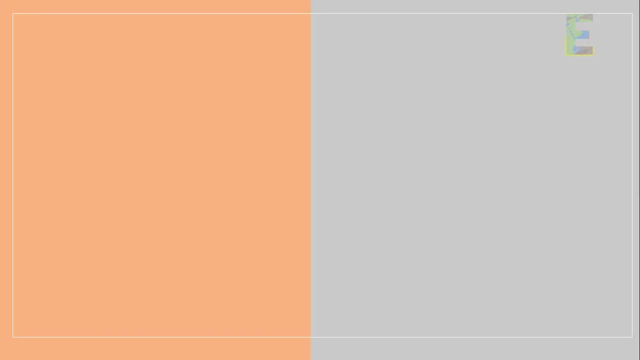 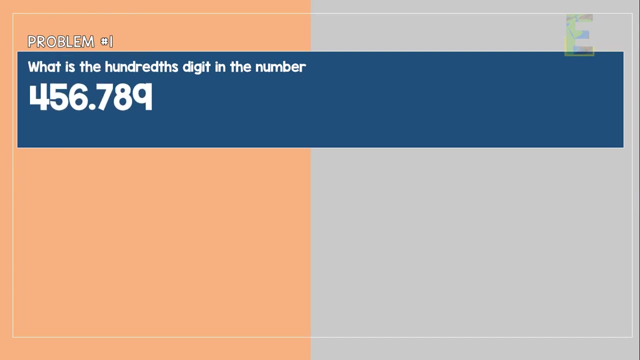 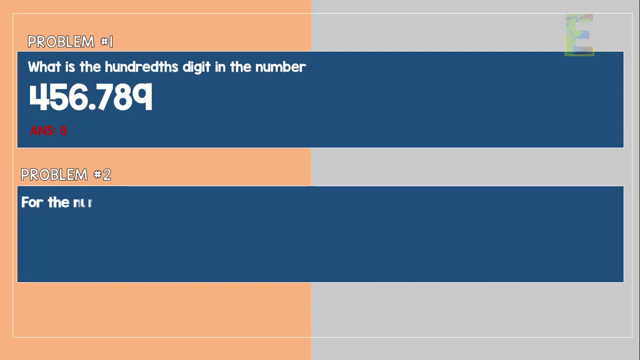 some problems. What is the hundreds digit in the number 456.789?? Correct, Digit 8 is in the hundreds place. therefore it is the hundreds digit. Hundreds digit is the second digit to the right of the decimal point. Now for the second problem, For the number. 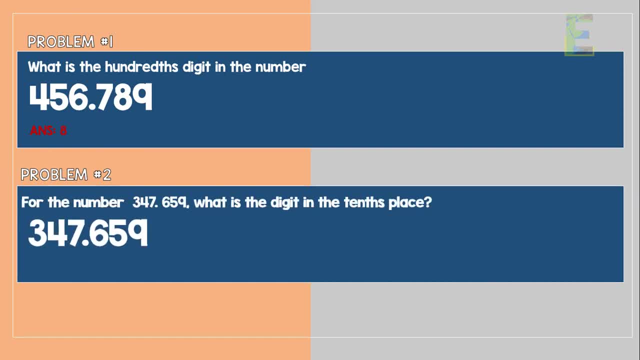 347.659,. what is the digit in the tens place? That's right. digit 6 is the digit in the tens place. Tens place comes immediately after the decimal point. Good job, you already know how to determine the decimal places and place value of a digit. 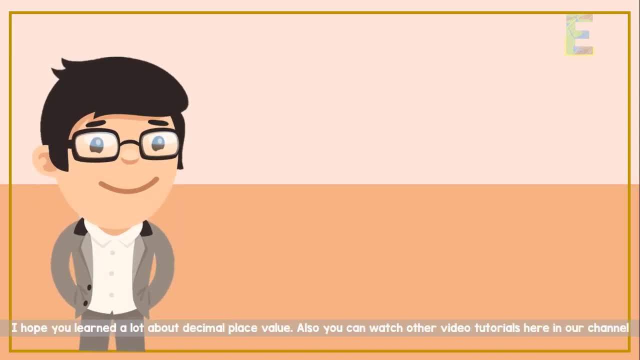 So that's it, guys. did you enjoy our topic for today? I hope you learned a lot about decimal place value Also, you can watch our other video tutorials here in our channel. Once again, this is EarthPen. Learning has never been this easy for anyone, anywhere. Have a nice day.